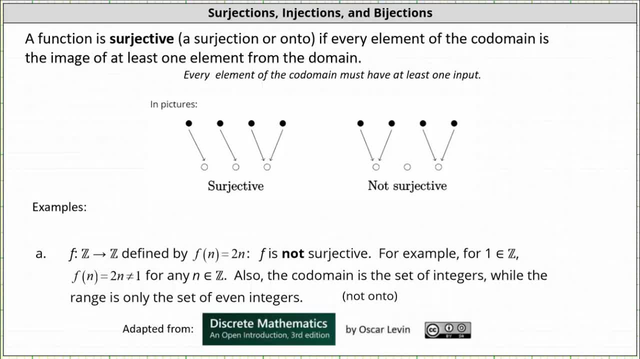 Welcome to a lesson on surjections, injections and bijections. A function is surjective, meaning a surjunction, or onto, if every element of the codomain is an image of at least one element from the domain. Or we can say, in order for a function to be surjective, every element of the 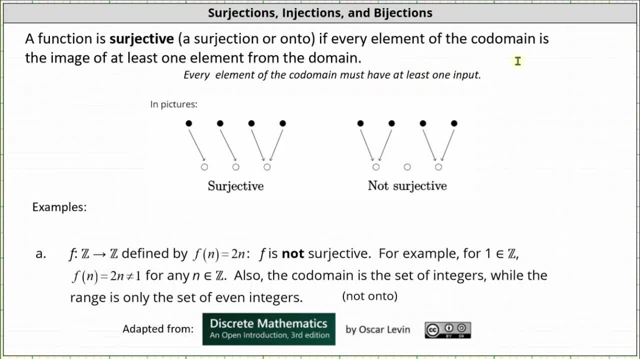 codomain must have at least one input. Looking at the mappings of the functions below, the function on the left is surjective. the function on the right is not surjective. The function on the left is surjective because the three elements in the codomain are images of at least one element from. 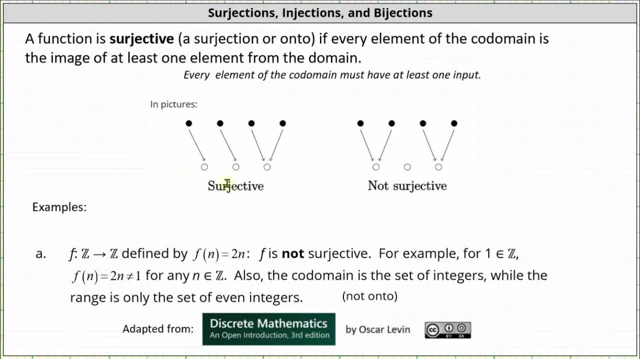 the domain. Notice, the first two elements in the codomain are images of exactly one element from the domain and the third element in the codomain is an image of two elements from the domain. This does satisfy the requirement that every element of the codomain 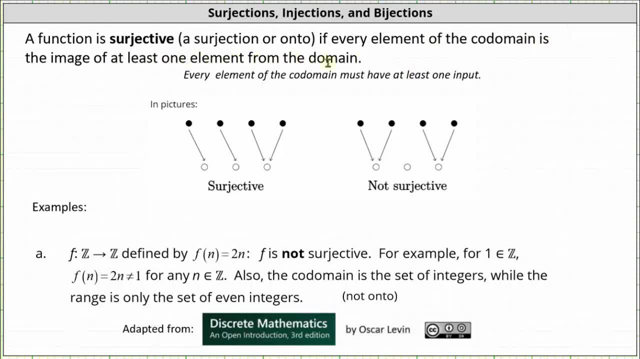 is an image of at least one element from the domain. At least one means one or more. The function on the right is not surjective because of this element in the middle in the codomain. It is not an image, or it's an image of zero elements from the domain. And now let's look. 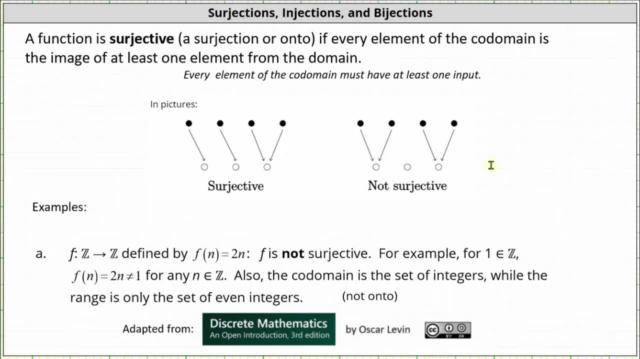 at three examples of functions and determine if the functions are surjective or not. First we have the function f, which maps the set of integers to the set of integers defined by f of n equals 2n. this function is not surjective. For example, 1 is an element in the set of integers. 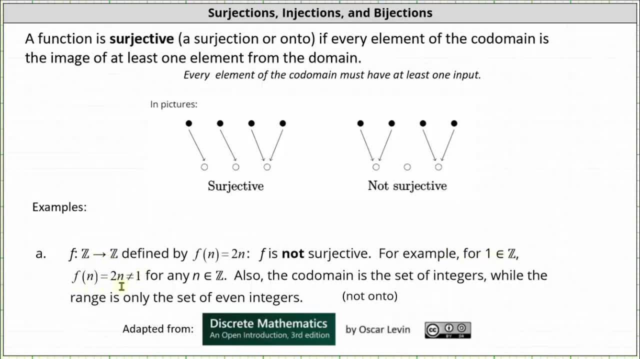 which is the codomain, and f of n equals 2n can't equal 1 for any n in the set of integers, which is the domain, which means all the odd integers in the codomain are images of zero elements from the domain. Also, the codomain is the set of integers, while the range 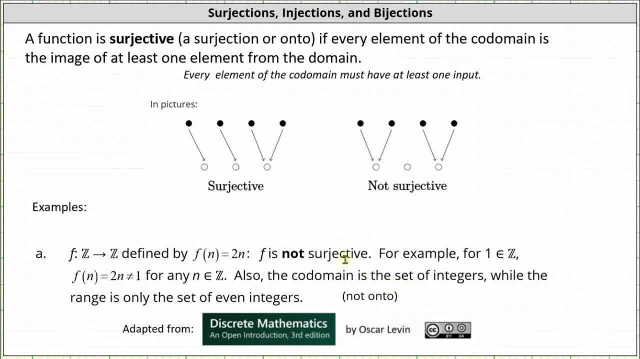 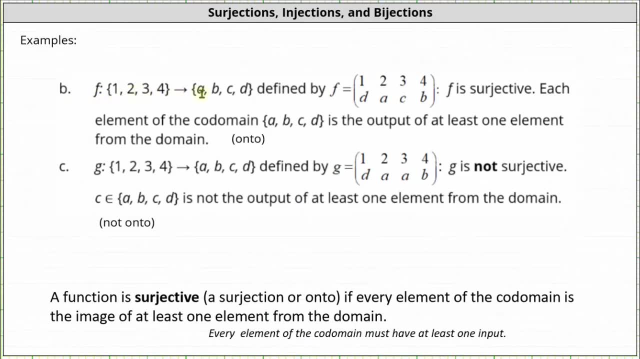 is a set of even integers, So the function is not surjective and not onto. Next we have the function f, which maps the set containing 1,, 2,, 3, and 4 to the set containing a, b, c and d, defined by f, given in two-line notation. 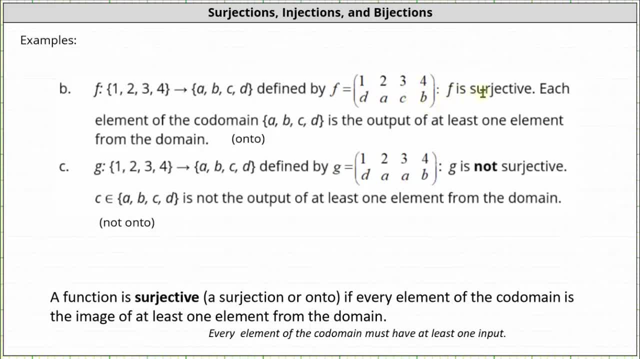 Analyzing the second rule of the two-line notation, f is surjective. Every element of the codomain, which is the set containing a, b, c and d, is an output of at least one element from the domain. Or again we can say: every element in the codomain is an image. 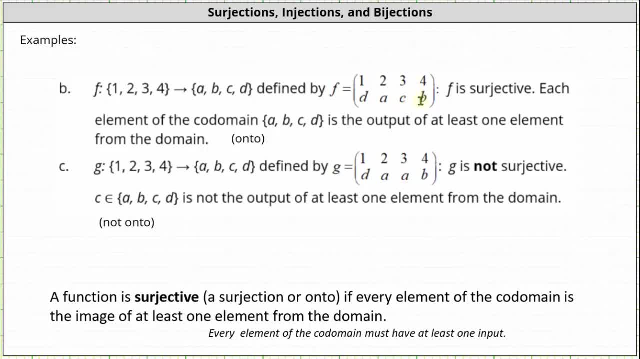 of at least one element from the domain. In this case, each element in the codomain is the image of exactly one element from the domain. So again, f is surjective as well as onto. And then we have c, which is the function g, which maps the set containing 1,, 2,, 3, and 4. 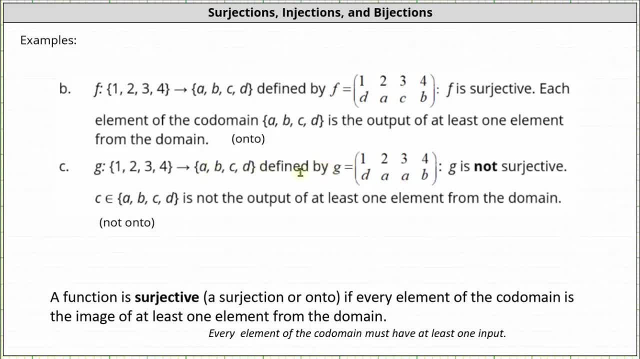 to the set containing a, b, c and d defined by, again, the two-line notation. Again, analyzing the second rule of the two-line notation, g is not surjective Notice. the element of c is in the codomain but it is not the output of at least one element from the domain. 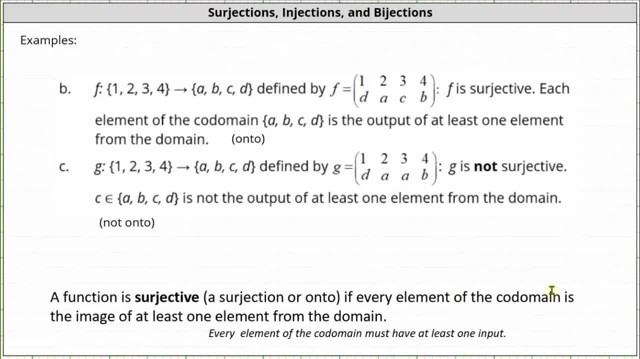 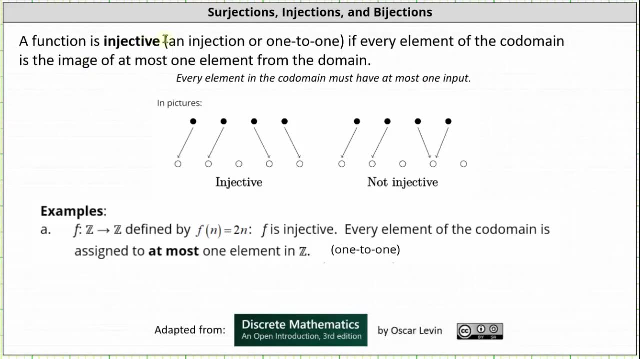 which indicates every element of the codomain is not an image of at least one element from the domain, because of the element c in the codomain, g is not surjective and not onto. And now let's define an injection. A function is injective or an injection or one-to-one. 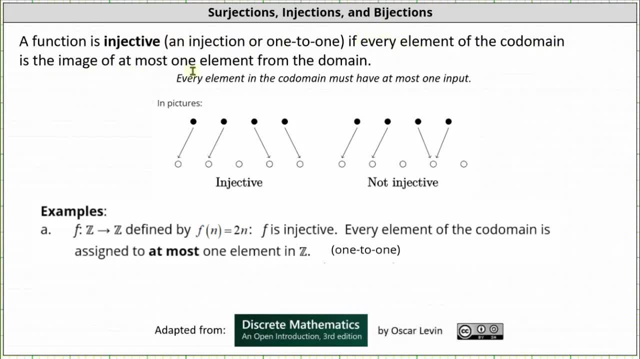 if every element of the codomain is the image of at most one element from the domain. So notice the change in language here. Here every element of the codomain is the image of at most one element from the domain. Or we can say: for a function to be injective, every element in the codomain must. 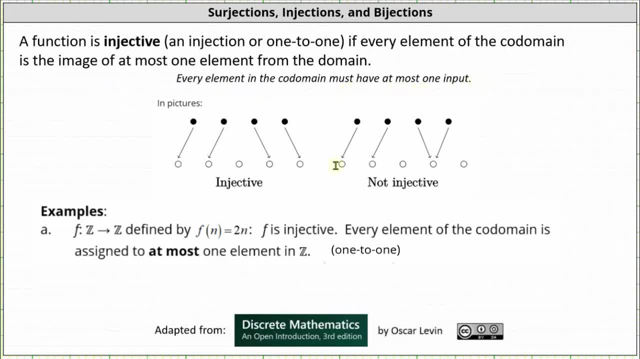 have at most one input. So again, looking at the two mappings below, the mapping on the left shows a function that is injective. The five elements in the codomain are images of at most one element from the domain. Four of them are images of exactly one element from the domain And the 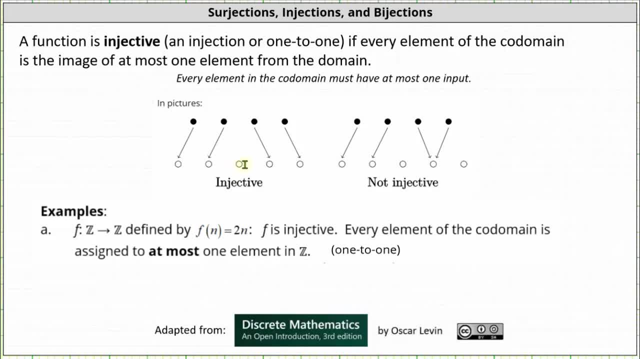 element in the middle. here is an image of zero elements from the domain and therefore the definition for an injective function is satisfied. The mapping on the right shows a function that is not injective because of this fourth element in the codomain. Notice this element in the 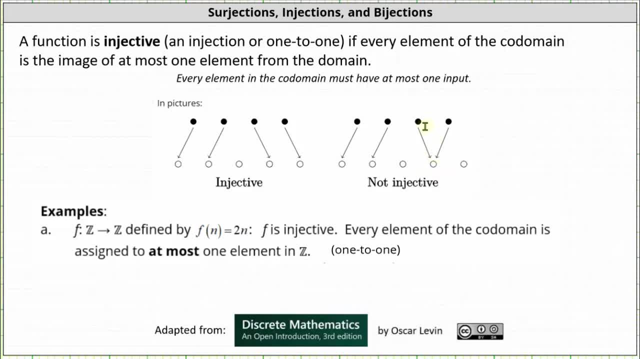 codomain is an image of two elements from the domain, which violates the definition for an injective function. Let's go through the same three functions and determine whether the functions are injective or not. So, again, going back to the first function given by a, we have the function. 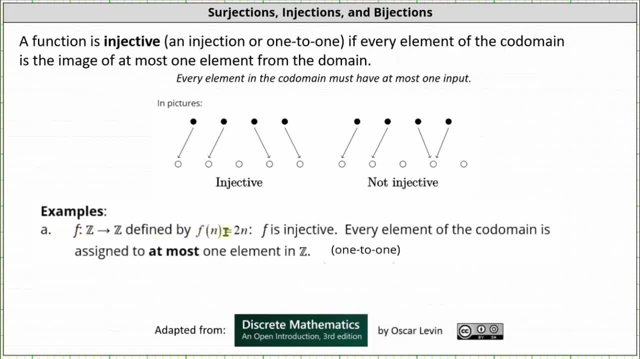 given by f of n equals 2n, where both the domain and the codomain are the set of integers, F is injective. every element of the codomain is assigned to at most one element in the set of integers, Or more specifically, all of the even integers of the codomain are images of exactly. 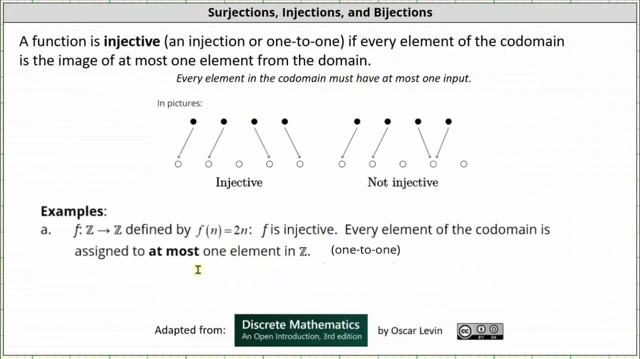 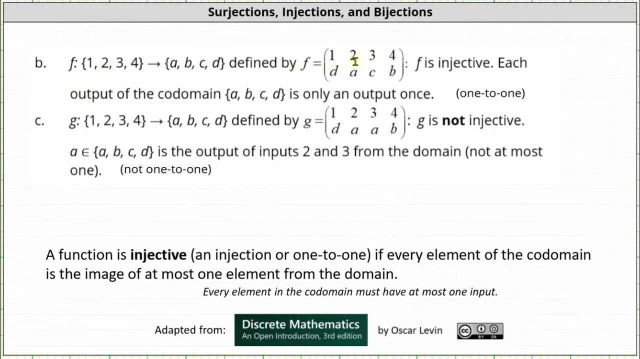 one element from the domain and all of the odd integers from the codomain are images of zero elements from the domain and therefore f is injective as well as one-to-one. Going back to part b, we have the function f given in two-line notation. 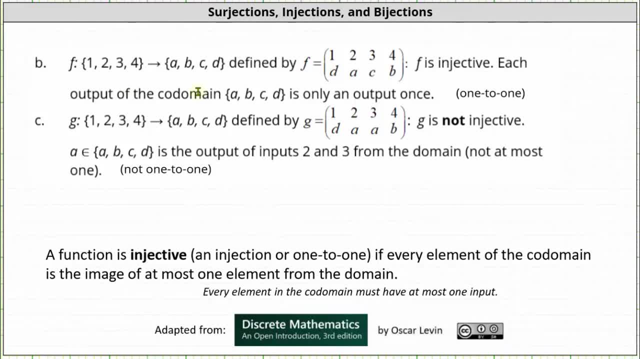 this function is injective. every output of the codomain, which is a, set, a, b, c and d, is only an output. once Or once again, every element in the codomain is an image of exactly one element from the domain which does satisfy the definition for an injective function. Again, 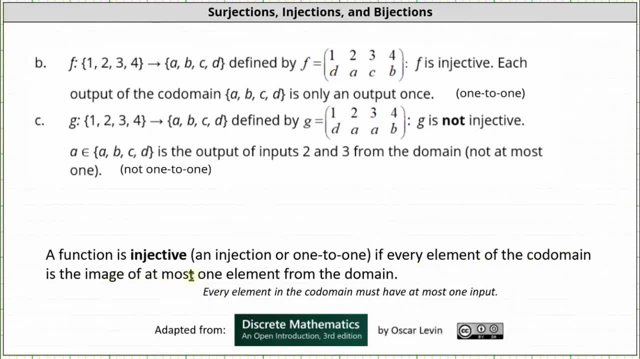 if every element of the codomain is an image of at most one, meaning zero or one elements from the domain, the function is injective. And then, for part c, we have the function f, given in two-line notation. the function g defined by the two-line notation, g is not injective. notice a is an. 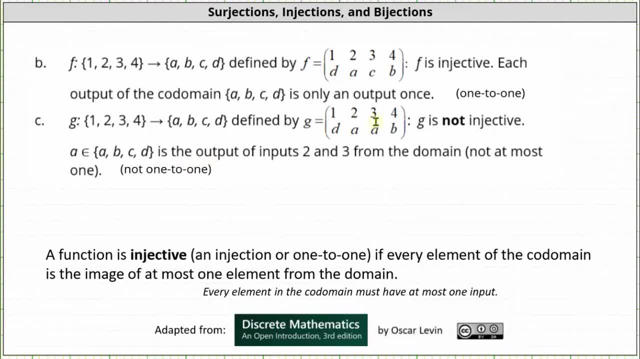 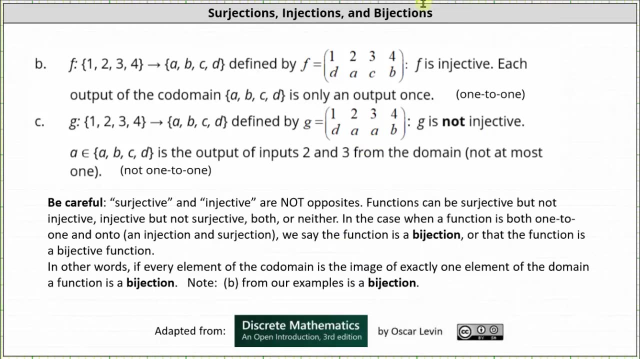 element in the codomain, but it is the output of the inputs two and three from the domain, which violates the rule of every element in the codomain being an image of at most one element from the domain. g is not subjective and not one-to-one We do need to be careful about. 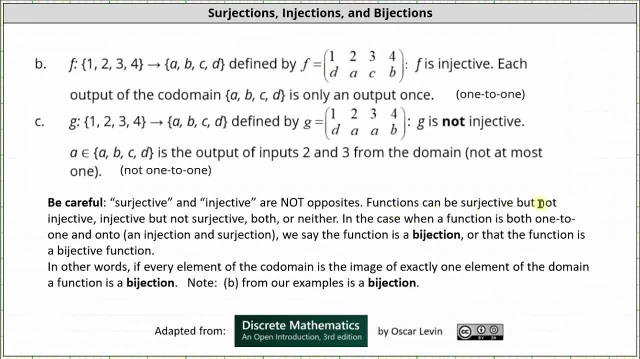 subjective and injective. they are not opposites. functions can be surjective but not injective, injective but not surjective, both or neither. In the case when a function is both injective and surjective, meaning both one and one, and onto. 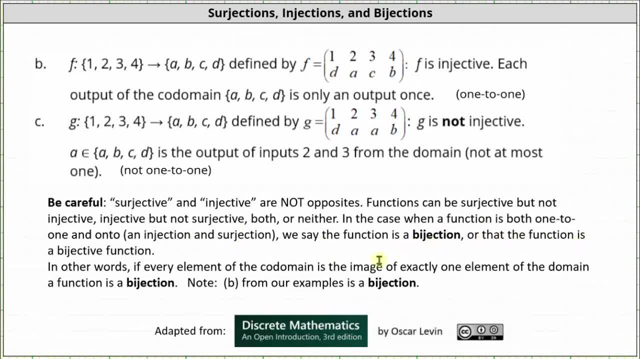 we say the function is a bijection or that the function is a bijective function. In other words, if every element of the codomain is an image of exactly one element of the domain, a function is a bijection. Notice: the function f given in part b is a bijection because it's. 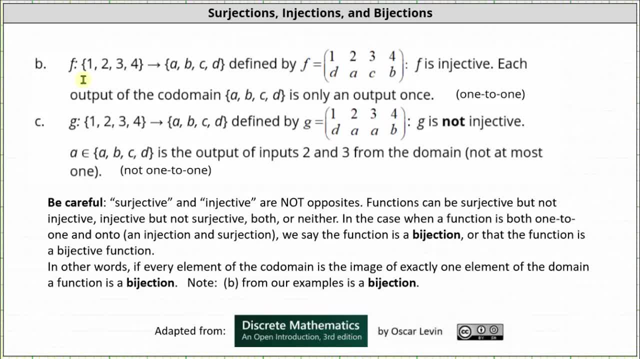 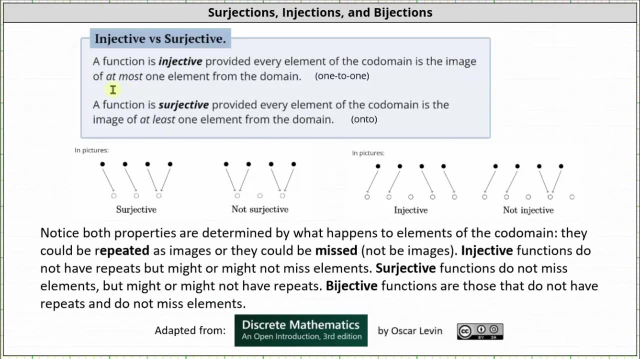 surjective and injective, meaning every element of the codomain is the image of exactly one element of the domain. And now let's compare the two definitions side by side. A function is injective, provided every element of the codomain is the image of at most one element from the domain.